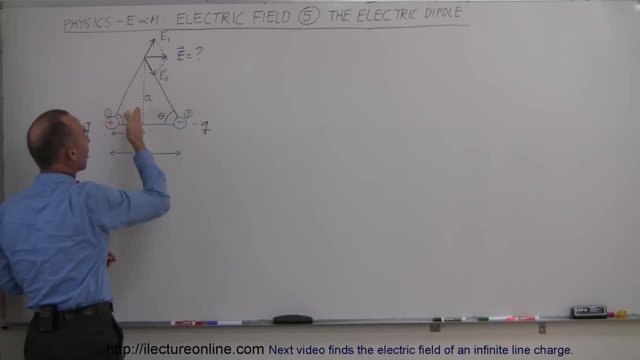 and we want to find the electric field at some point along the what we call perpendicular bisector. so what we find is we find the halfway point between the two charges, which is right here. we draw a line perpendicular to that line and then we want to find the electric field somewhere. 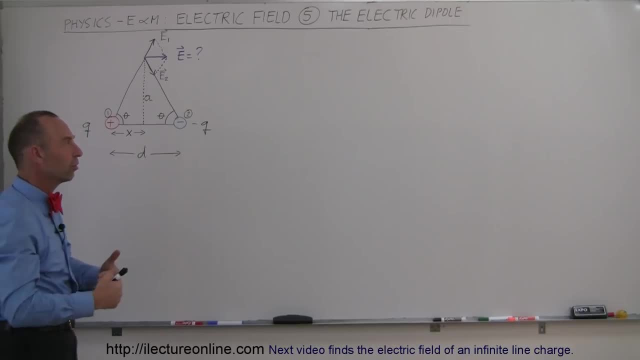 along that line. so we're going to do things kind of in a general sense and then when you throw numbers in there, you just kind of, just you know, do it exactly the same thing, but with numbers. all right, so what do we do here? well, you can see here that 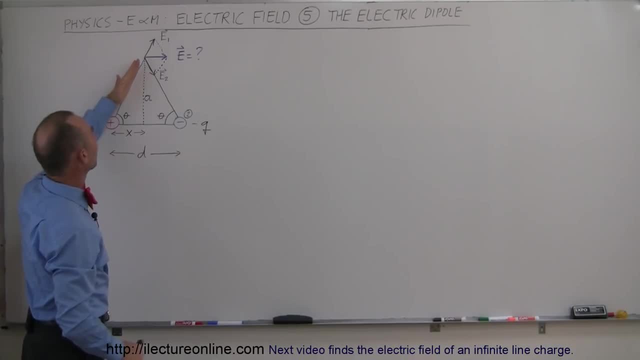 based on this charge, right here we're going to have an electric field that emanates in this direction, and so we're going to call this port right here, the electric field at this location, due to this positive charge. then we know that for negative charges, electric fields are directed. 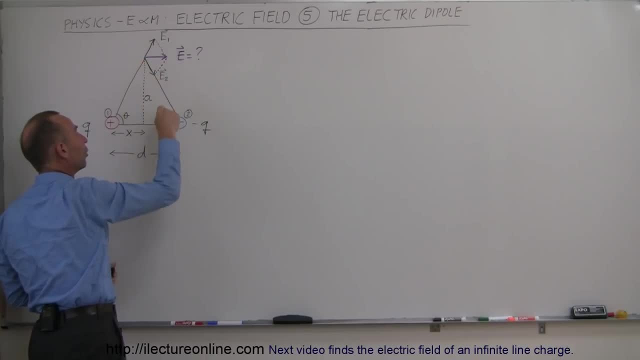 towards the charge, so the electric field at this very same location to this charge is in this direction, and so the total electric field experienced by both of these charges at this location will then be to the right, which is simply the way we're doing this. we're going to draw the 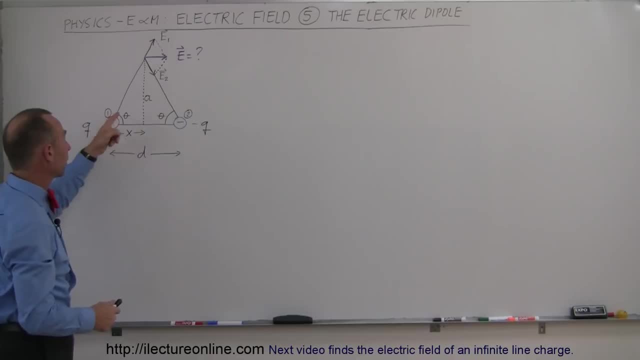 a vector sum of E1 and E2.. I call this charge 1, I call this charge 2, as the note data right there Notice. the difference between the charges is d. therefore x is half the distance between them, The distance from the line connecting the two charges to the point of interest right there. 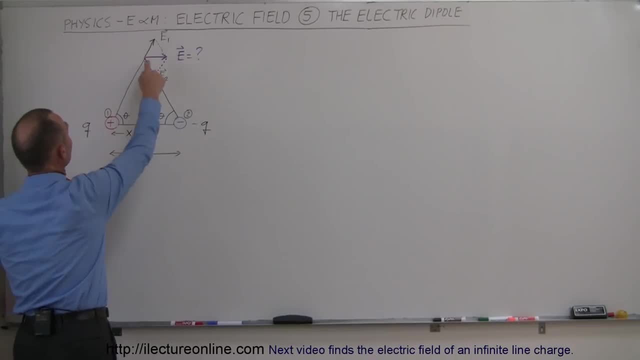 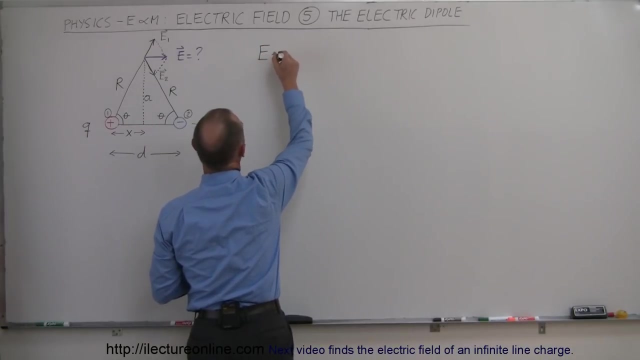 is a, and so that makes this distance right here. from that point to this charge and from that point to this charge, that is equal to the distance r. Okay now the general equation to find electric field due to a point charge is this: electric field is equal to k times q the charge. 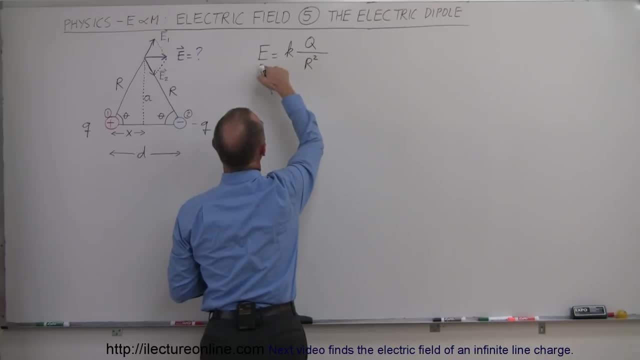 that causes it divided by the distance from the charge to the point of interest, r, and we square that. so that's a general equation. So to find E1, we could say that E1, in this case, is equal to k times q divided by r squared. and we can say that E2, therefore, also, is equal to k times q divided by r squared. 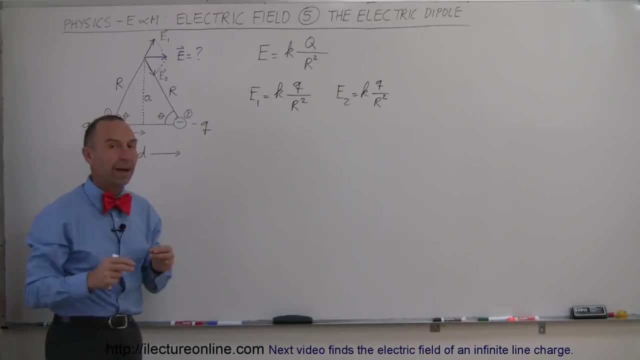 Now notice that I did not put the negative in there, because I didn't care about the direction. I only care about the magnitude of E1 and E2.. Now, in order to add those two, I can see that the vertical components of E1 and E2 are simply going to cancel each other out. Notice that if I draw 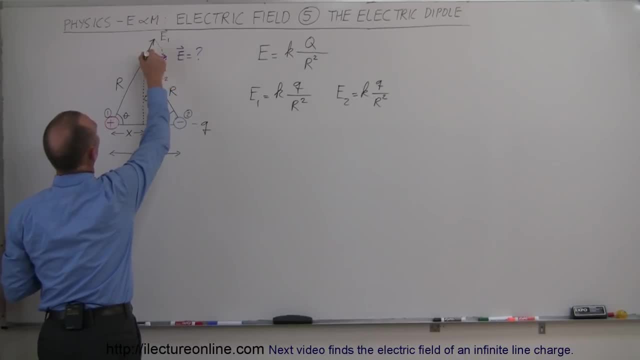 that let me use some green here. so here you can see that would be the horizontal component of E1 and the vertical component of E2 and the horizontal component of E1.. vertical component of V1.. Here's a horizontal component of V2 and a vertical component of V2.. 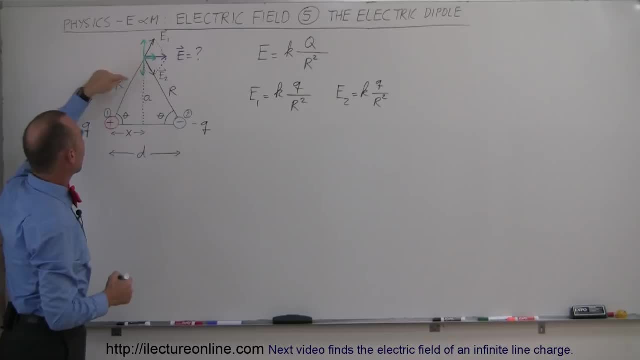 And notice that, because of their distance from that point to each of the charges is exactly the same and the size of each charge, the magnitude of each charge, is exactly the same, except one is positive, one is negative. you can see that the vertical components should be equal in size. 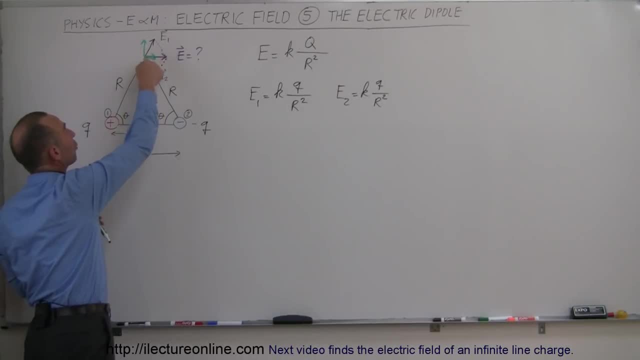 and therefore cancel each other out, and the only surviving components are the two horizontal components which we need to add. So how do you find a horizontal component of V1 and E2?? Well, if I assume that this here is the angle theta, I can then see that this here is the angle theta. 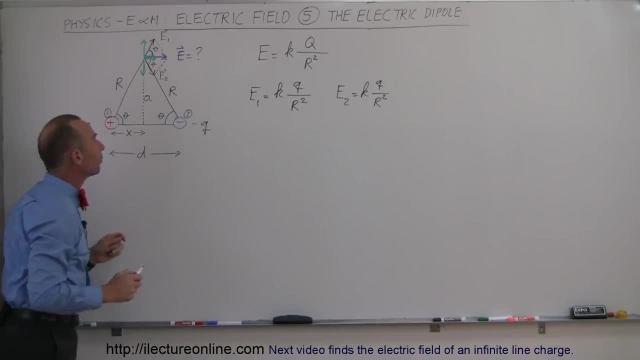 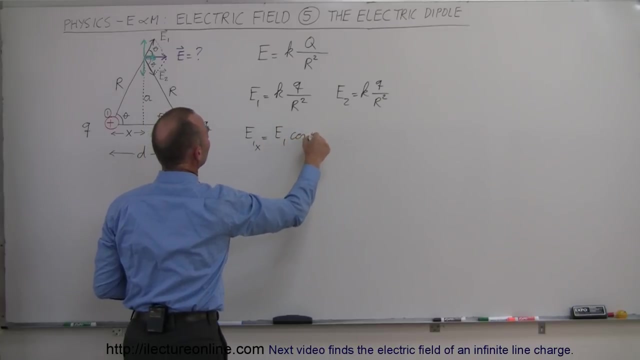 as well. and then here this should be the angle theta as well. So that way we can see that the horizontal component is simply going to be the magnitude of V1 times the cosine of that angle. So we could say that E1 in the x direction is equal to E1 times the cosine of theta. Now remember: 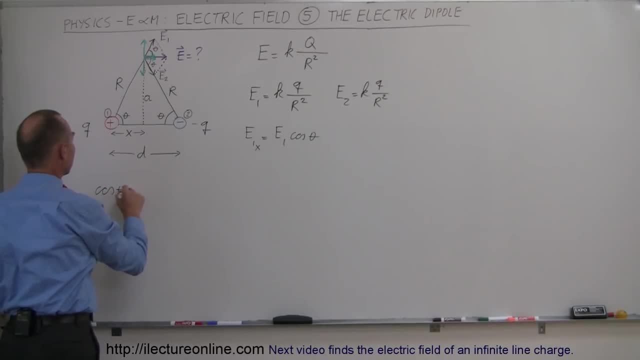 the definition of the cosine of any angle is the ratio of the adjacent side divided by the hypotenuse. So if we look at this angle right here, which is the same as this angle, there the adjacent side would be x and the hypotenuse would be r, So that means it's equal. 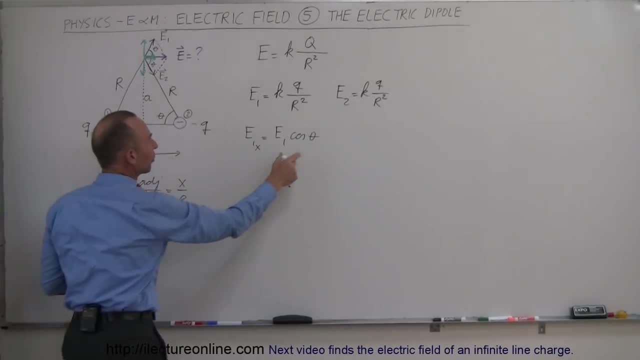 to the ratio of x divided by r, and I can then replace the cosine of theta by the ratio of x over r. Now, also, in this particular picture, I can also say that r is equal to the square root of the adjacent side squared, and the opposite side squared right here, So it would be x squared. 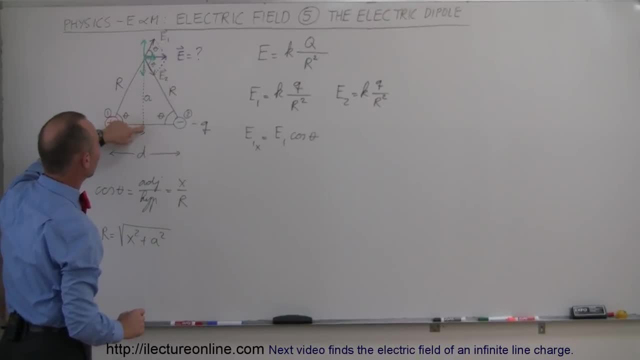 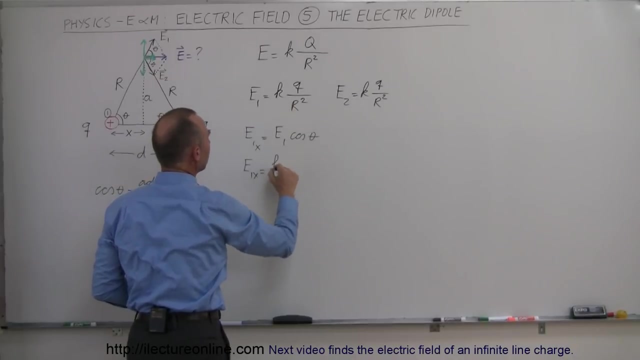 plus a squared A, of course, is simply the distance from the bisector. I mean not from the bisector but from the line joining the two charges to the point of interest. All right, so if I then plug that in here, notice that E1 in the x direction is equal to E1, which is k. 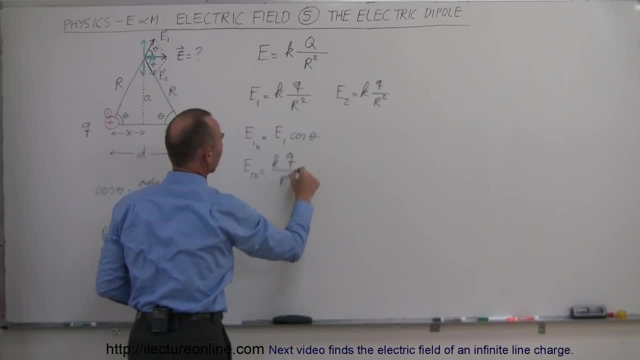 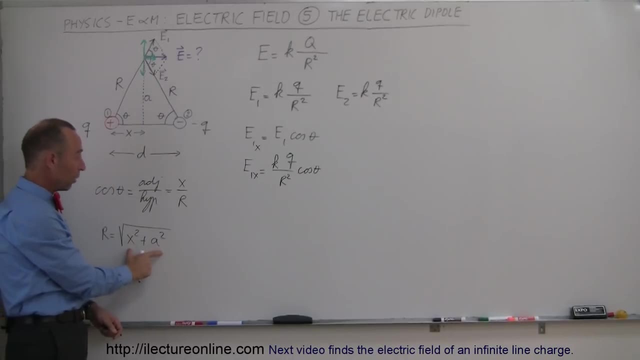 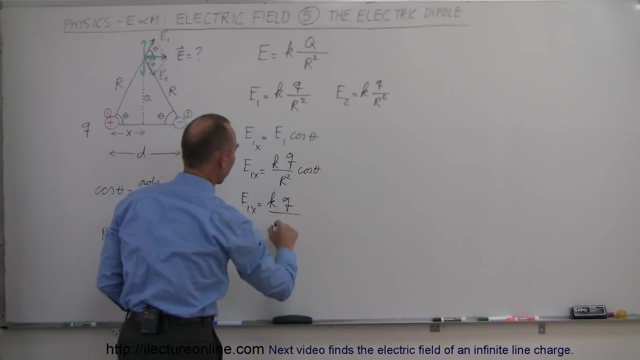 times q divided by r squared times, the cosine of theta. Now I can replace r squared by this right here. So if I square r I get this quantity squared, or simply what's underneath the radical. so this is: E1x is equal to k times q divided by. let's see here x squared plus a squared times. 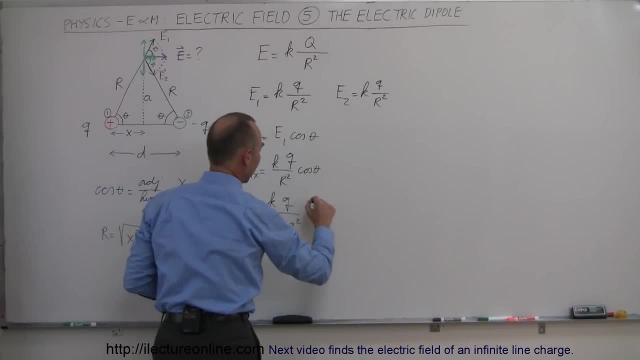 the cosine of theta, which is x over r, So that would be x divided by r, and then again this r can be replaced by this right here, and so we then get: E1x is equal to kqx over x squared plus. 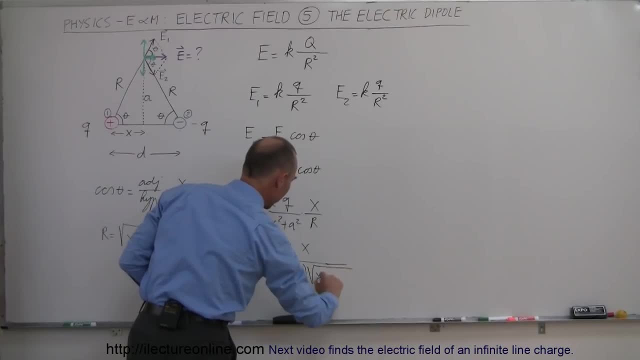 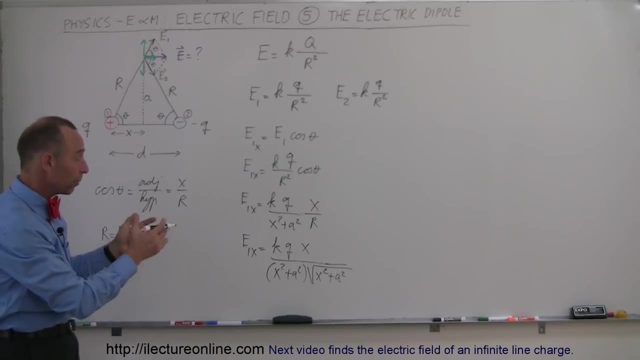 a squared, and the whole thing multiplied by the square root of x squared plus a squared. So finally, if I combine those two, when I multiply them out, I get the denominator raised x squared plus a squared raised to the three-halves power. 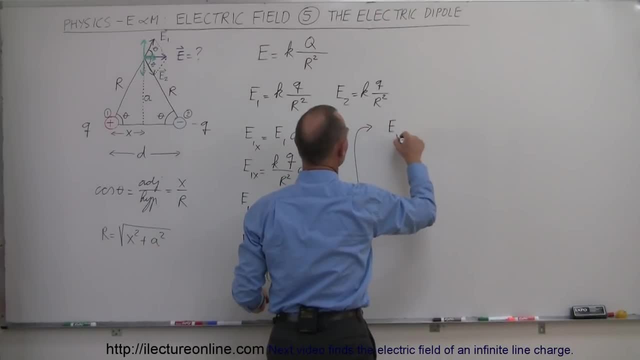 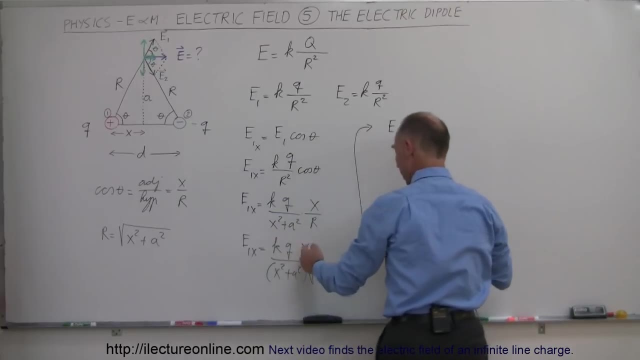 So what I can do here? I can then say that E1x- nope, I forgot my one- it was already right in the x. So E1x is equal to: right here we have kqx divided by this quantity. right here, x squared. 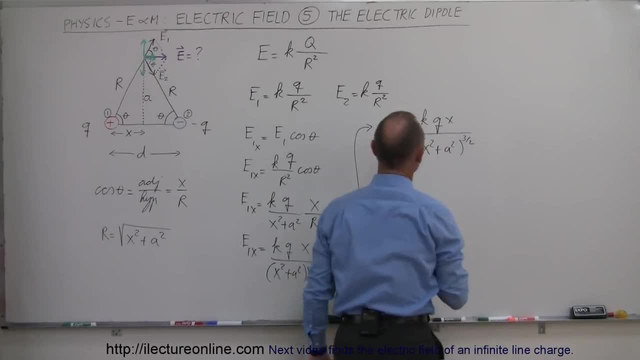 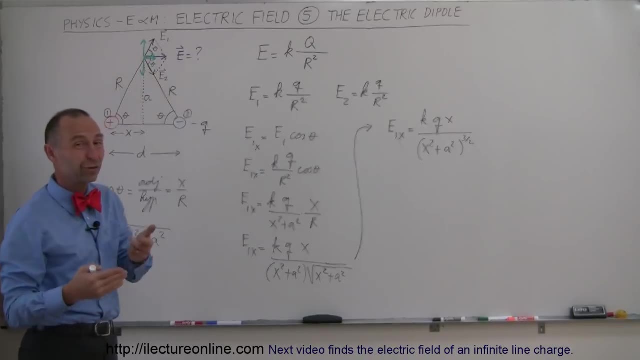 plus a squared to the three-halves power. Alright, so that's E1 in the x direction, and because of the symmetry here we know that E2 in the x direction should be the exact same amount, so we can say that E2 in the x direction therefore also is. 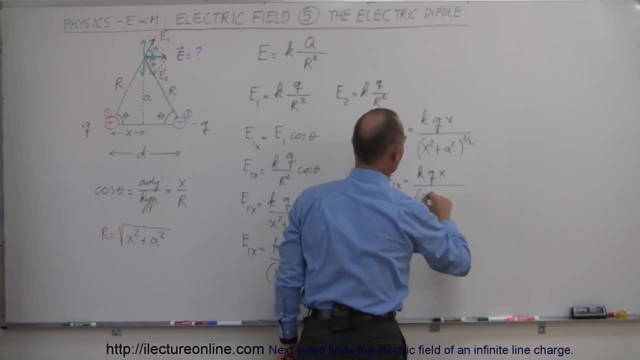 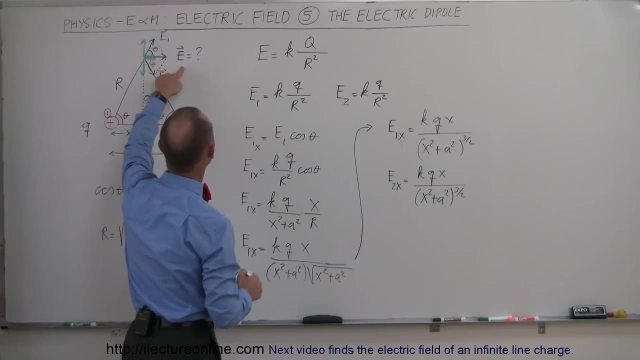 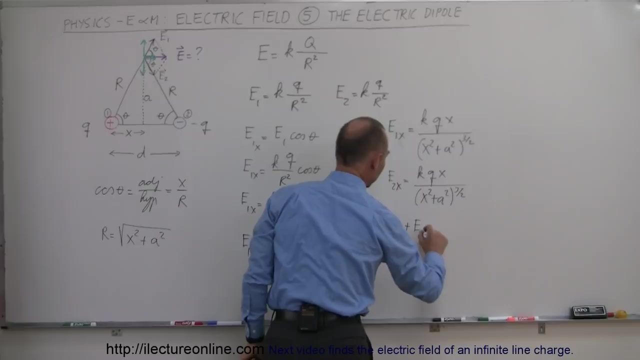 kqx divided by x squared plus a squared to the three-halves power. And then, of course, we can then see that E is simply the sum of the two x components. so E is equal to E1x plus E2.. And so therefore, that's equal to twice this number, so two times kqx divided by x squared plus a. 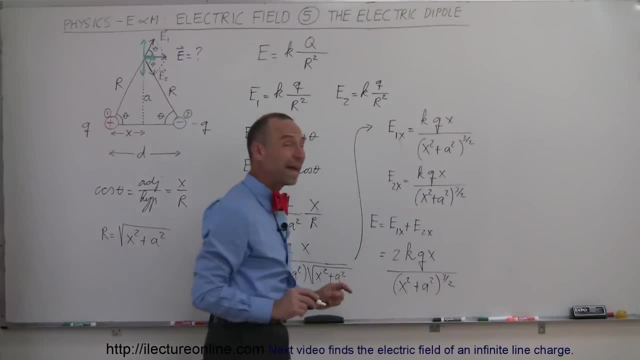 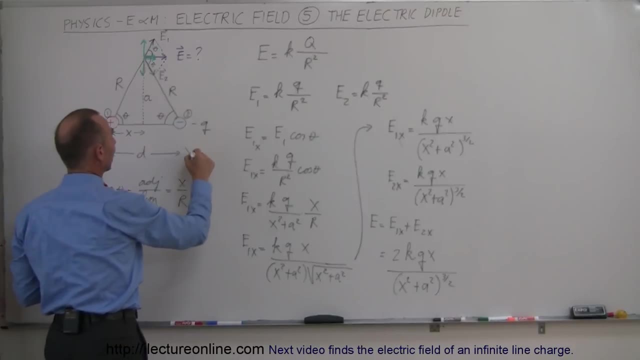 squared to the three-halves power. Now going back to what x was equal, to remember that x was just half the distance between the two charges. so in other words, we can say that x is equal to the distance between the two. 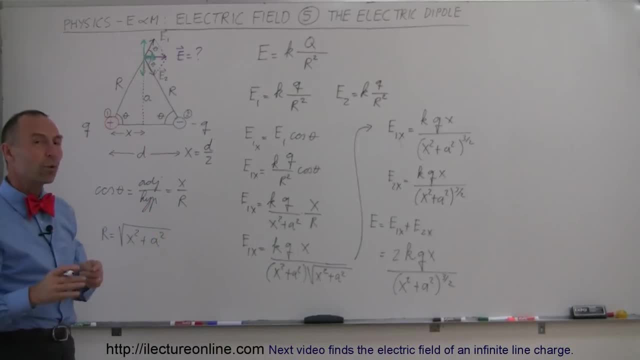 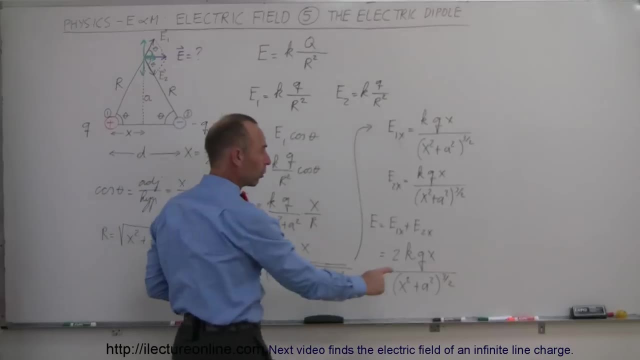 charges. So we can say that x is equal to the distance between the two charges divided by two. And most likely when you work with dipoles you want to express the answer in terms of the distance between the two charges, not half the distance between the two charges. so we're going to replace 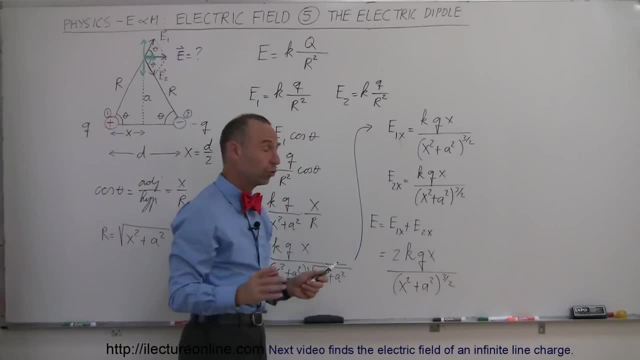 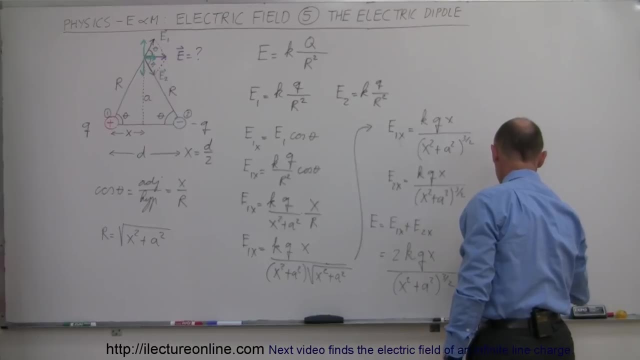 the x by distance over two and x squared by distance over two. So what we'll get there then is that the final answer will be: well, not quite almost there: 2kq times d over two. divided by d over two, quantity squared plus a squared to the three-halves.